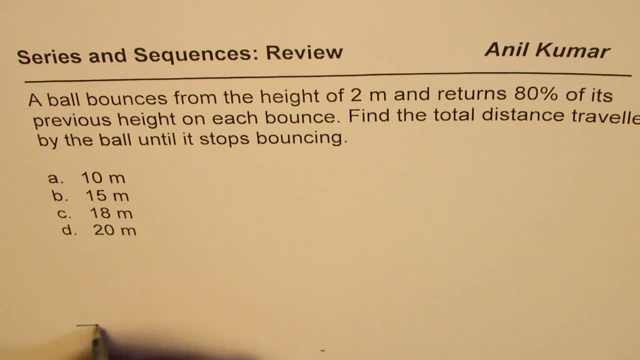 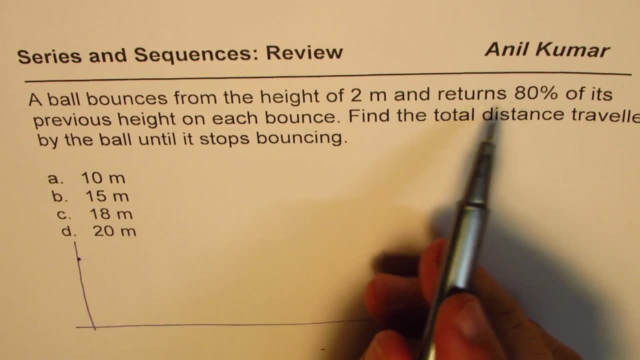 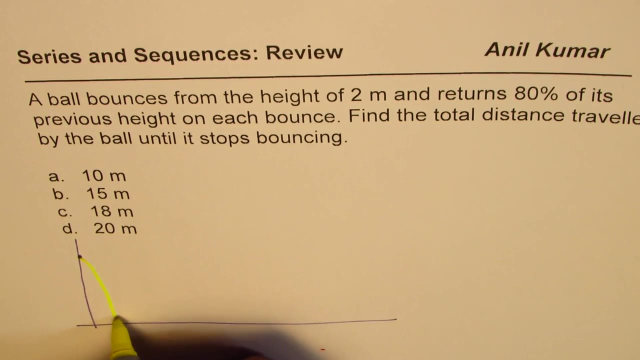 Look into my suggestions. Okay, let's think about it. So let's say that's the ground and the ball is bouncing from this place, which is two meters high. So let me show the path of the ball. Let's say the ball falls here and then bounces and then goes back to 80%- right, not the full amount- and then again bounces and then goes to 80% and then again comes down, goes to 80%. 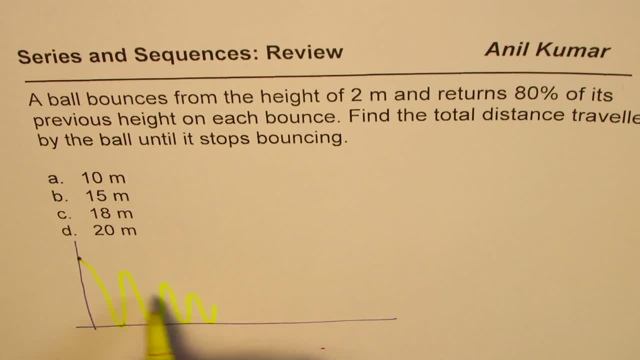 Then comes down and let's say, this process continues. So every time it bounces back, let's say it started with a value which is given to us as two meters. right, So it is two meters. and next time it will be at a height which is 80% of two meters, That is, two times 0.8, right, And then next time be two meters. 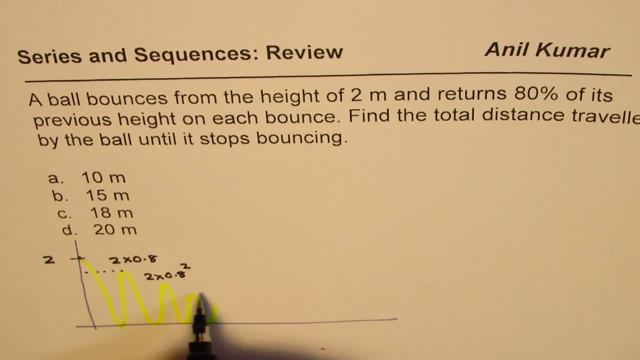 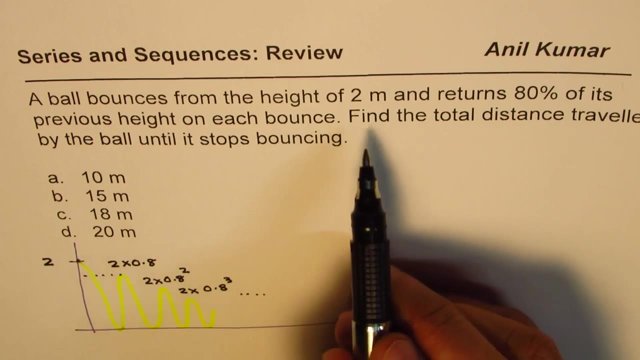 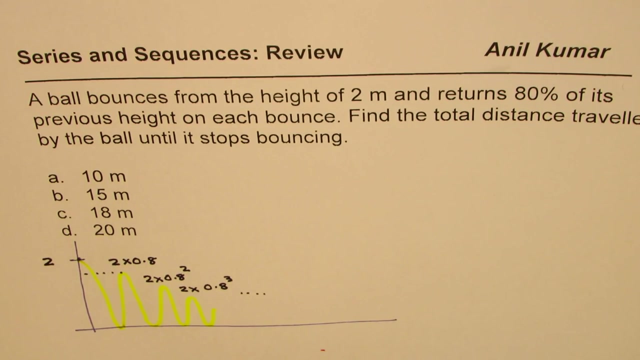 That is two times 0.8 square, and then be two times 0.8 cube, and so on. right, So that is going to be the height after each bounce: 80% of its previous height. Find the total distance traveled by the ball until it stops bouncing. You can still pause the video, answer the question and then look into my suggestions. 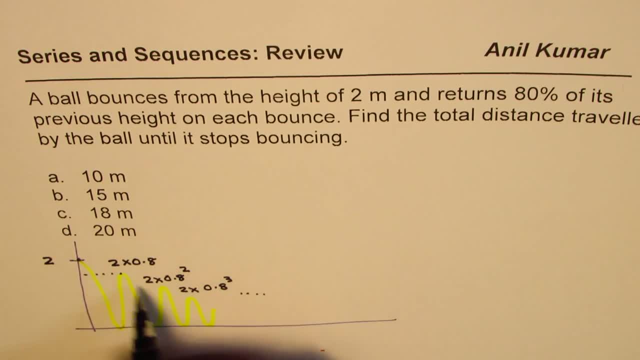 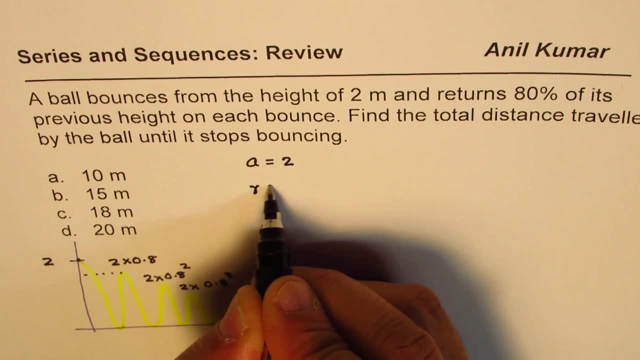 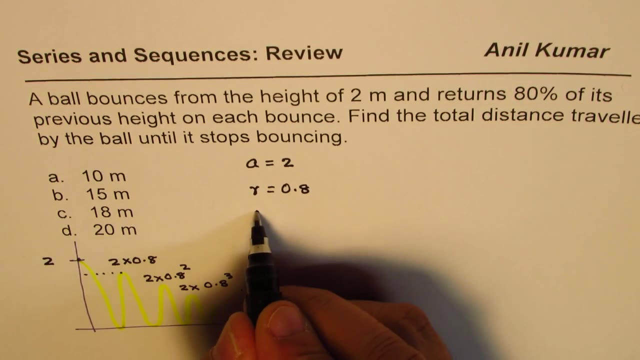 Well, now let me give you an example, Let me give you the formula. So you know this is a geometric series, right So, where we know it starts at two right And r is you're getting multiplied by 80%, which is 0.8, and sum of this is an infinite series, right, So n, where n approaches infinity because it stops bouncing, So it will almost at infinity, will be equals two. 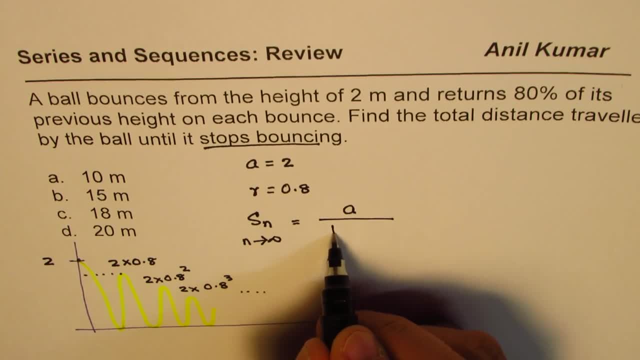 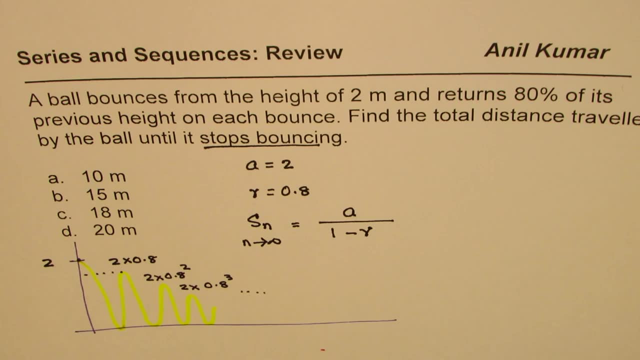 So you know this is a geometric series, right? So n, where n approaches infinity because it stops bouncing, So it will almost at infinity- will be equals two, Starting from a, 1 minus r. So that is the formula for solving this question, right? So you can use this formula, answer the question and then we'll look into further. 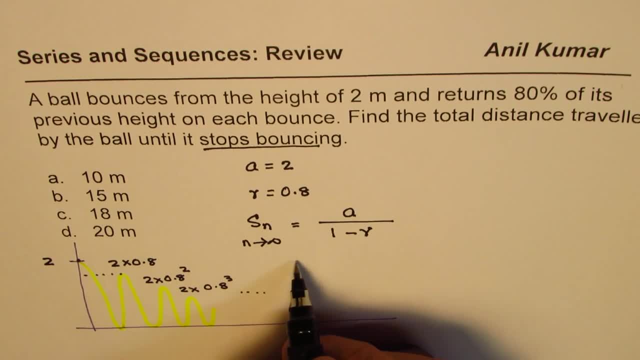 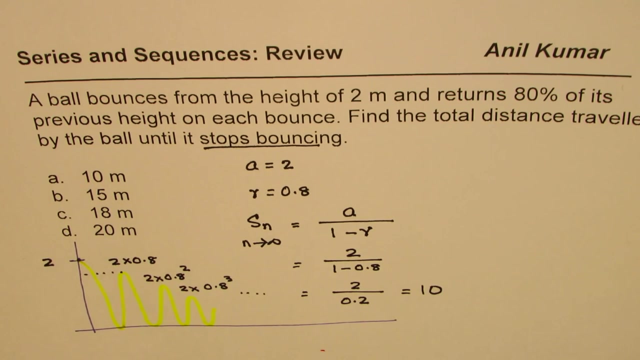 Okay. So if I apply this formula, what do I get? 0.2, and that is equals to 10.. So this is what we get. We do have 10 in one of the options, but is it the right number? Now think about it. Pause the video and then answer the question. I hope it is very interesting. 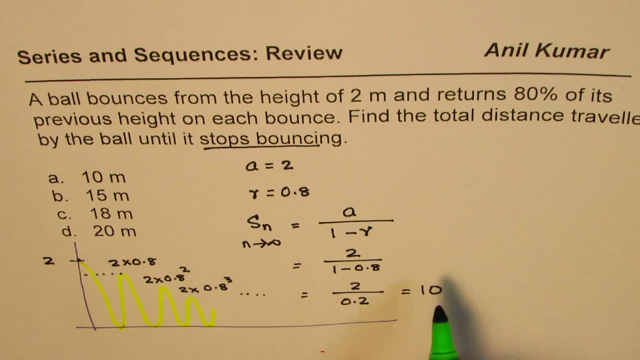 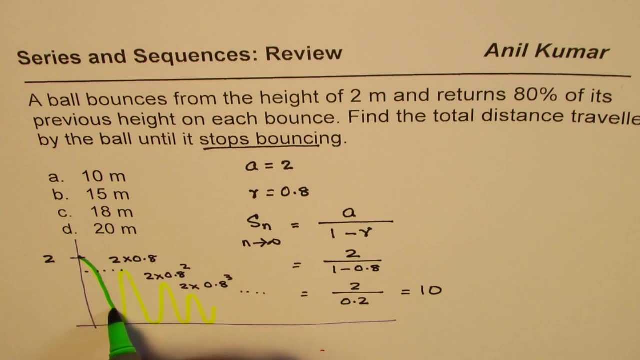 Now let me tell you further. Now, this 10, which is sum of these numbers, actually is talking about. we're counting only one number, Okay, Okay, While it is getting dropped off, right. So we have just counted these portions. Do you see that? Now, in this series, when we add it, we have added only the distance of falling, but the rising distance has not been counted. Do you see that? 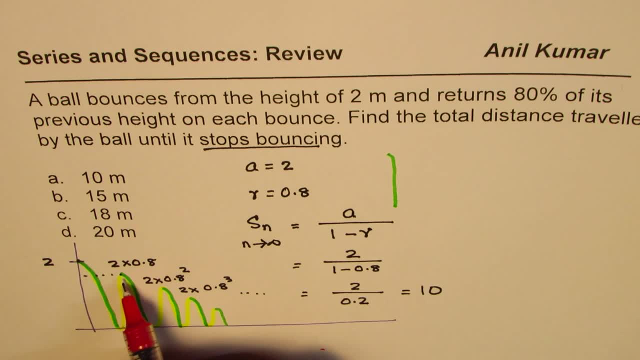 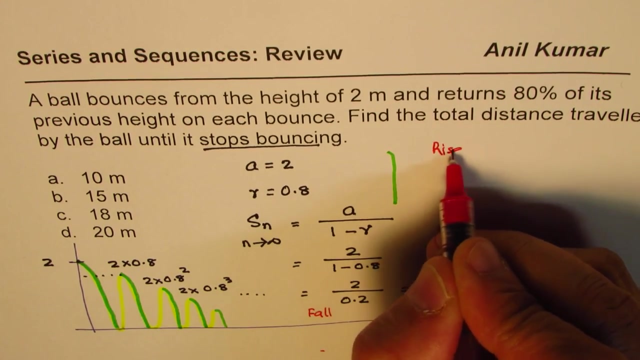 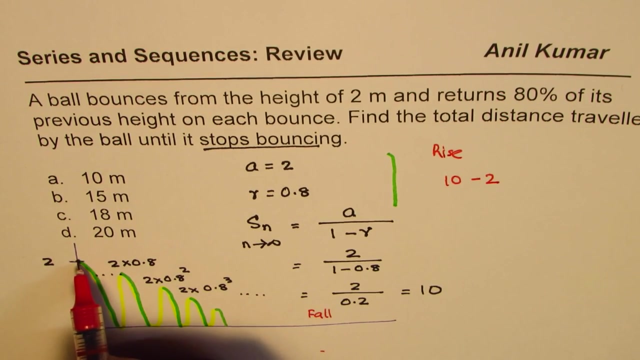 After every fall there is a rise by the same distance, correct, Except for the first one. It starts at 2.. It does not rise to 2.. But after that, whatever distance it falls, it has already risen to that. So falling distance is followed by the rising distance. So this is falling distance, total fall. And how much does it rise by? It rises by 10, take away 2.. Since it did not rise 2, right? Do you see that It falls only 2.. 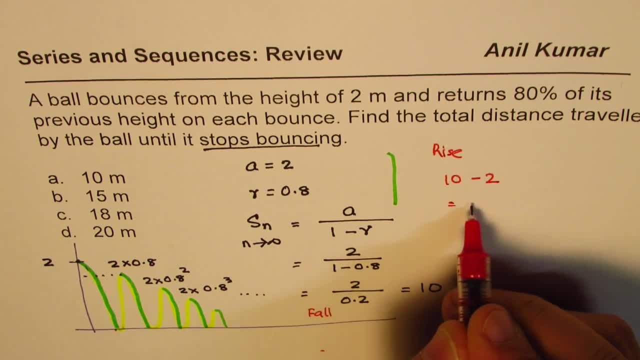 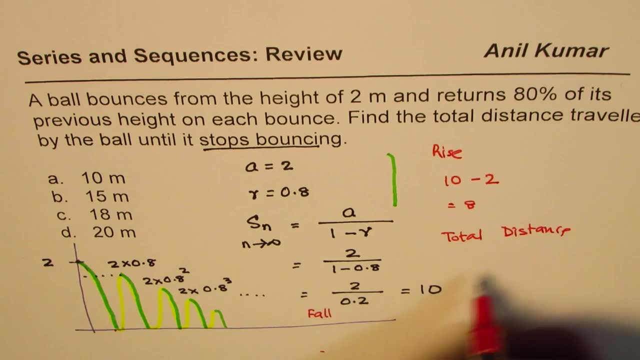 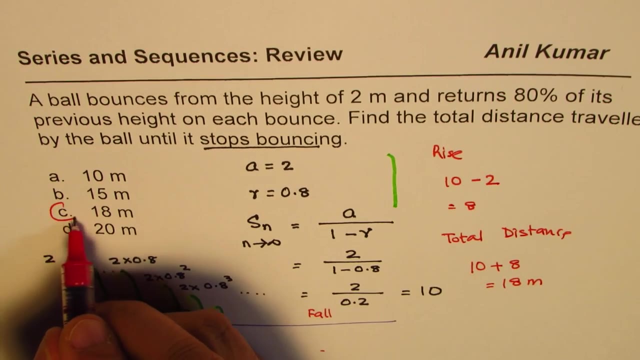 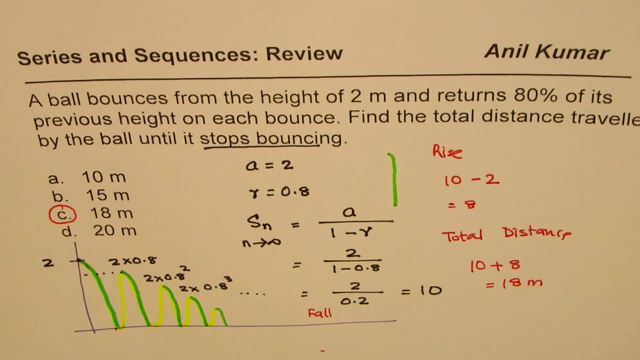 Okay, So 10, take away 2, it rises, which is 8.. And therefore total distance is: how much Is 10 plus 8,, which is 18 meters? So the option C is the right option. I am Manil Kumar and I hope you find it very interesting. It is one of the most important questions from this unit on sequences and series. 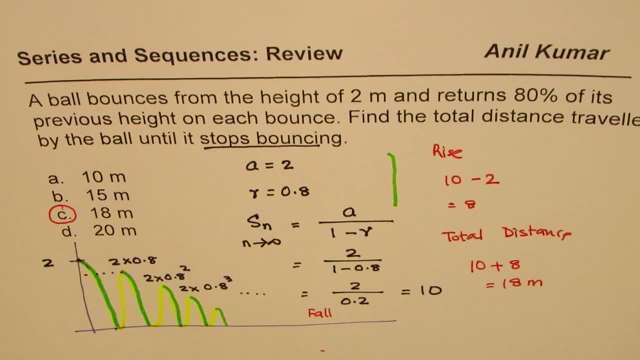 Okay, Okay, Manil Kumar, you can always pause, look into this suggestion and then think about it. Thank you and all the best.